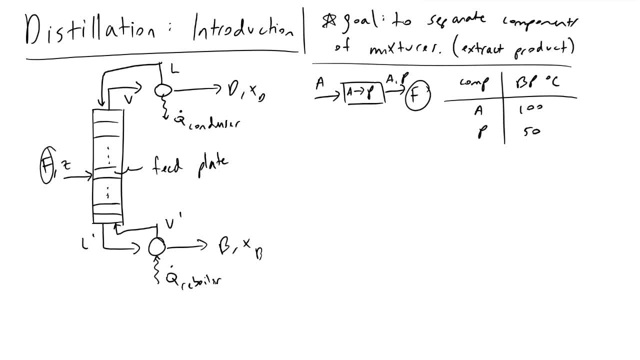 going on at a distillation column. I think it's best to start at the bottom and then examine what happens as we ascend the distillation column. And so what we're going to find is that at the bottom tray the heavier component is concentrated, And the reason for this is because we have a liquid that is descending our column. 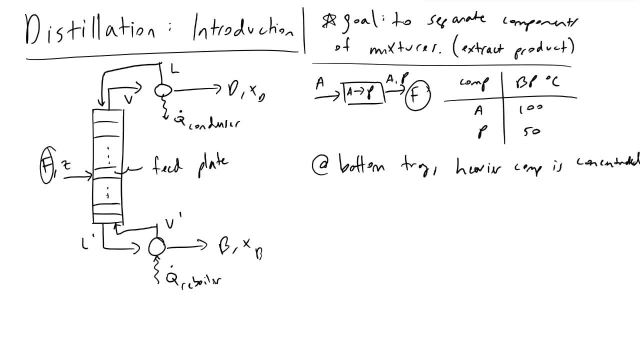 and the heavier component, component A, is more likely to exist in that liquid phase that is for our distillation column, And so when we reach the bottom tray of our distillation column, it's going to be very concentrated in our heavier component, which is our reactant called A. 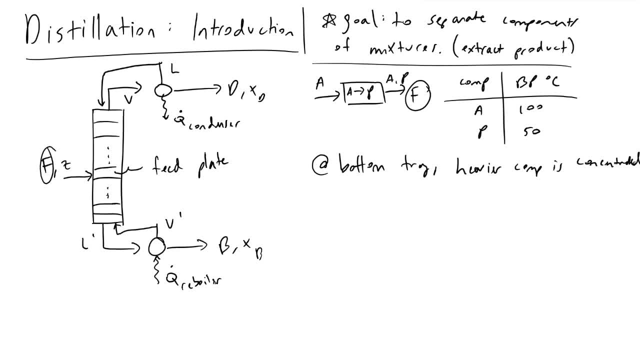 And so, once we enter the bottom tray, what will happen is we're going to be having a heater here, We're going to have some kind of reboiler, and in practice this would just be a copper coil and we would be running electric current through it, for instance. or perhaps we're burning methane and 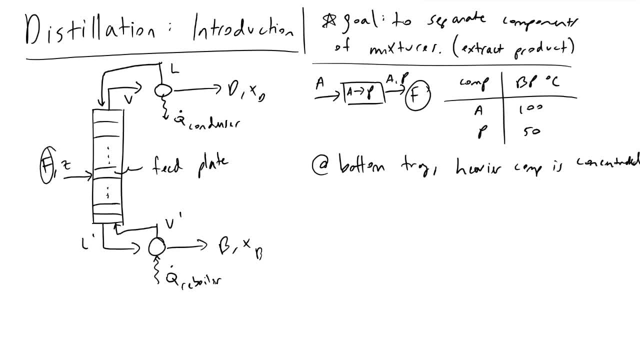 having a fire. But the point is we're supplying heat into our bottom plate and as we heat this mixture that just entered the bottom tray, some of it's going to vaporize, And the part of it that vaporizes is going to exist. more likely it's going to have your lighter. 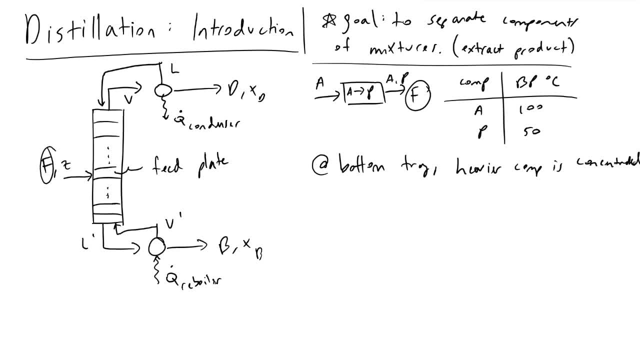 component in it, But you're also going to have some of your heavier component, And so we are going to vaporize this. We're going to get V prime, which is a vapor phase that is going to go back up into our distillation column, And V prime will be somewhat concentrated or will have a higher concentration. 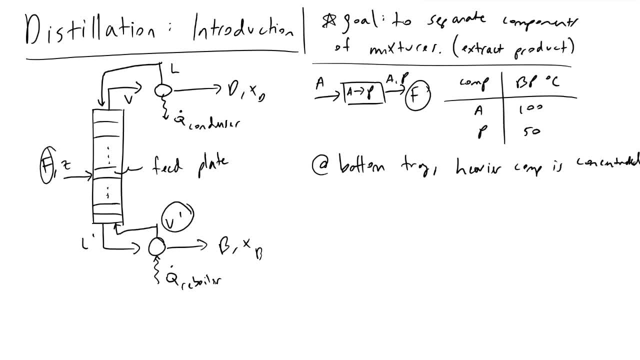 of your lighter component, our product P, than did the liquid phase that entered. It is very important to note that at each tray we reach a vapor-liquid equilibrium, And what this means is we've given sufficient residence time for the two phases to reach equivalent chemical potentials, And this is 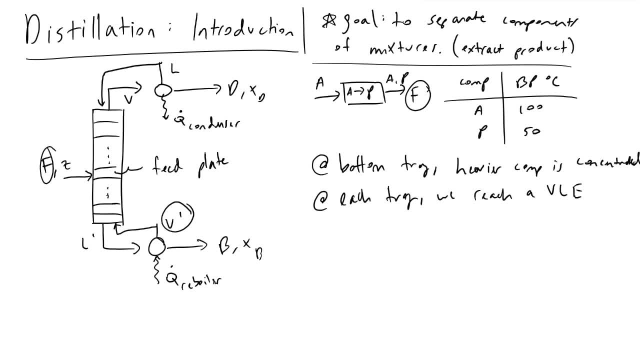 thermodynamic lingo, But what it really means is that we have allowed whatever wants to exist in the vapor phase to vaporize and enter the liquid, the vapor phase. And whatever wants to stay in the liquid phase can stay in the liquid phase And we've given them enough time to they can do. 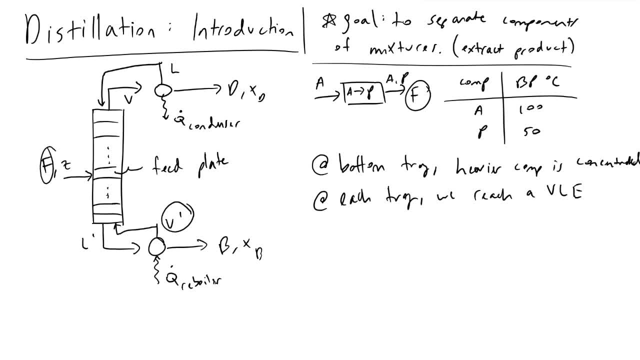 that, And that is how we are separating our mixture- is by relying on this temperature difference between our two components, And so this is a temperature difference between our two components, And so this is a take-home message for distillation columns. It revolves almost entirely around this difference. 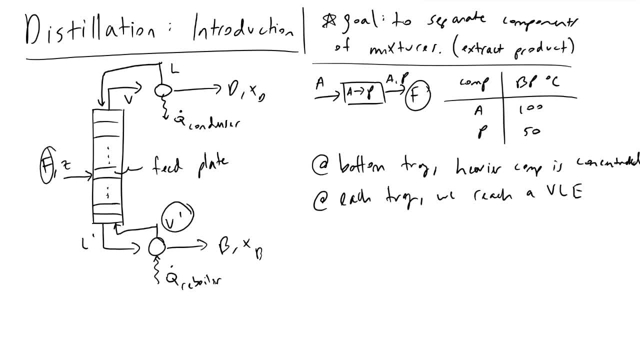 in boiling points between species that we have in an effluent stream that is entering our distillation column from a reactor. And so with this information, this vapor phase V prime that we've just sent back up into our column is now going to enter into another plate, Another. 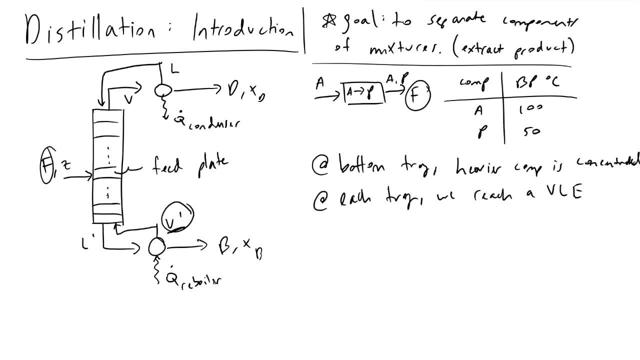 area in which we're going to reach vapor-liquid equilibrium again, And as we ascend the column, each tray is progressively cooler, And so as we move to the next tray, we're going to have more vapor-liquid equilibrium, which is barely crab-like to begin. 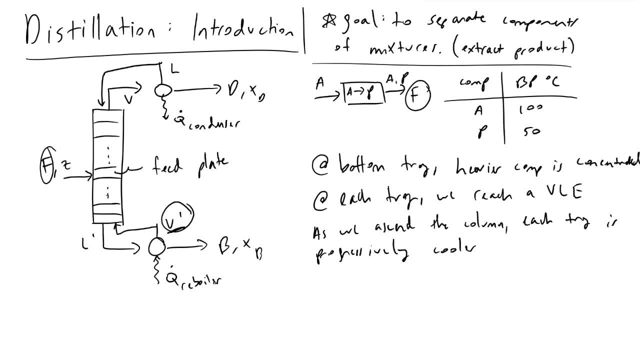 with To give it a Brad туwh claws to, based on what you've, Jayne, and he're going to be able to measure and calibrate it. One of the most essential things you're going to want to remember is when we come to the top of the roots of the iOk thread. the showed that the vapor-liquid equilibrium is going to be significantly lower than previous temps, And because 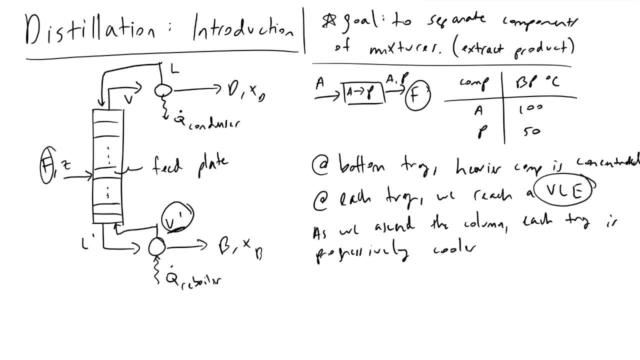 reach this vapor-liquid equilibrium at each tray as we move up our column And depending on the number of trays that we have, we can get better and better extraction, But we do get diminishing returns, And this is modeled in some very important equations And we can see this when we are working. 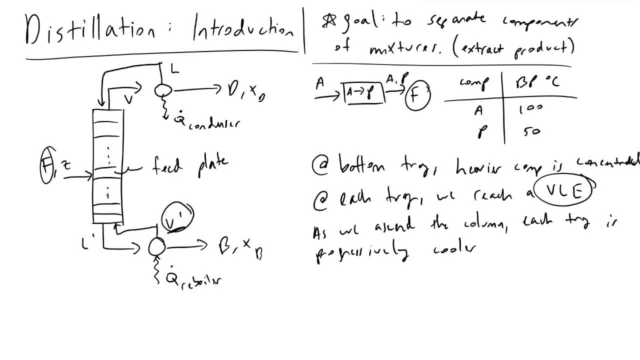 with solutions or mixtures that have azeotrope compositions, And so, to continue with this discussion, what we'll find is that we're going to have a temperature gradient. A temperature gradient must exist to have mass transfer, And what that means is that if you're operating a distillation column, in practice 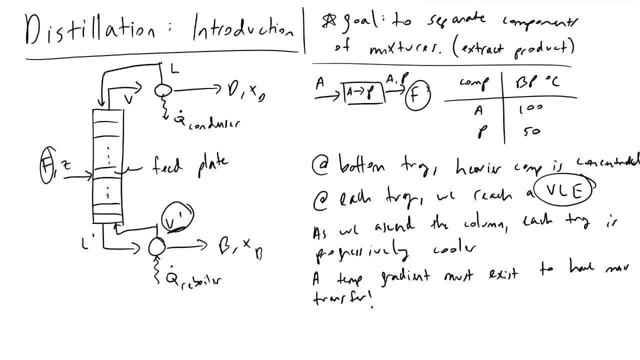 and you are seeing that each tray is the same temperature. that's a bad sign because that tells you that you're not getting any better extraction by having more trays, And more trays means you're paying more money and you're having to supply more energy in your reboiler to operate your distillation column. 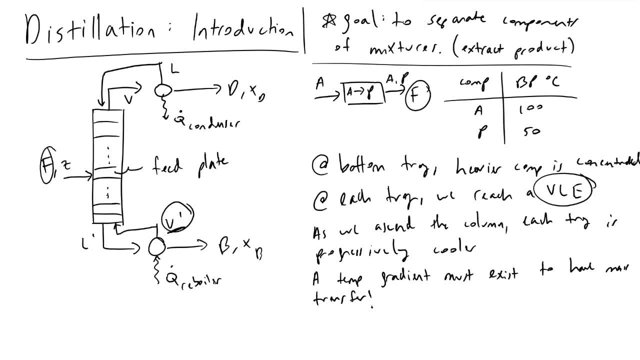 and so you have an inefficient process And so you need to go back to the drawing board, change the number of trays you have, lower your reboiler duty before you realize a nice temperature gradient, And so to kind of get a back of the envelope calculation as to what kind 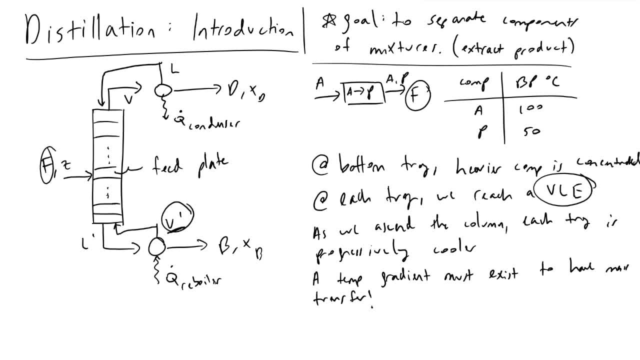 of temperature gradient you would expect in this binary system that we're working with, with our unreacted reactant A and our product P. we would expect that this reactant A would be able to get an extra volume from this冷est, or at least a certain amount of temperature of the two trays that. 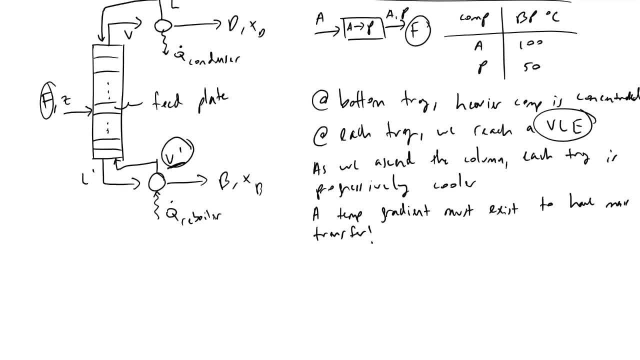 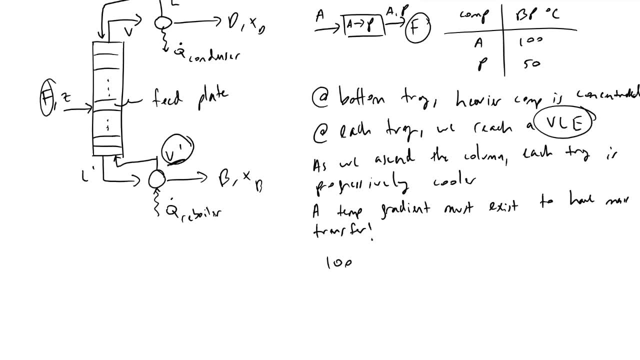 we would have in this series. With that we would be able to kind of get a back of the envelope. calculation P: we would expect to find a temperature gradient like this. So it would take the boiling point of A, so we'd have 100 degrees C minus 50 degrees C divided by 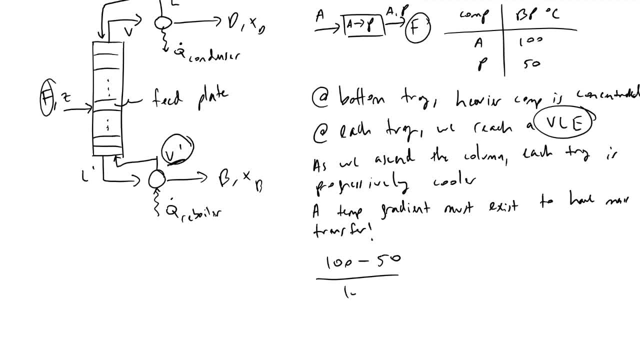 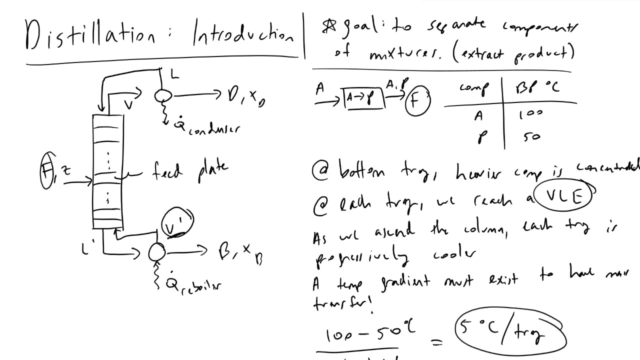 and if we had 10 trays in our distillation column, we would expect to see that our trays would have a 5 degrees C temperature gradient per tray, And in other words, what this means is that it's 5 degrees C colder for each. 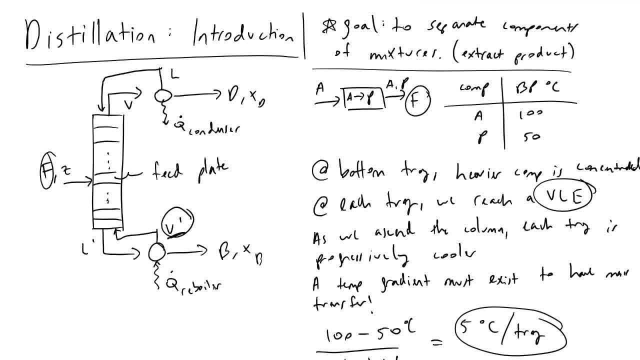 tray working with this binary system. And so working with binary systems is nice because I can do this kind of calculation. You can get an idea of what kind of temperature gradient you want to see, But it gets quite a bit more complicated when you're working with multi-component systems. 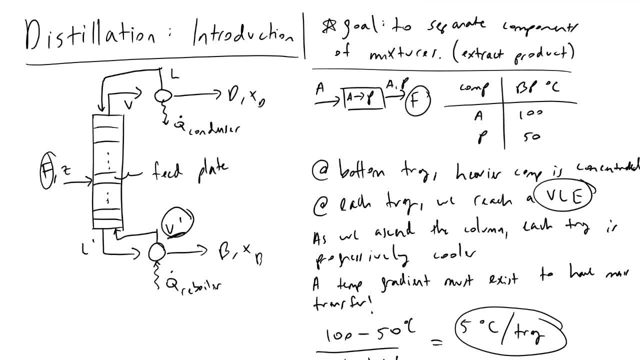 more than two components, But for the sake of an introduction, this binary system gives us an idea that we're going to want to see if we had a distillation column with 10 trays and we had two components and the boiling points of each component was independent of pressure And 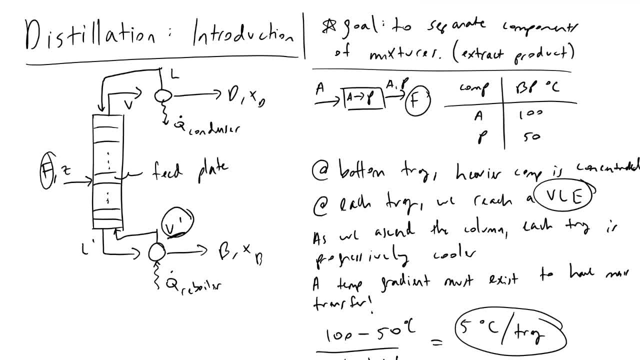 quite often the pressure difference is negligible or has a negligible effect on the boiling point. Then we can say that we want to see a five degrees C temperature drop as you ascend the distillation column at each tray, And so this is a very important note, just so you have an idea. 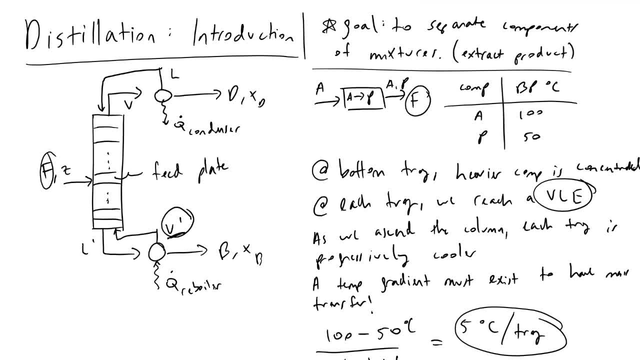 And this what will happen is at each tray, the colder temperature will get us a new vapor-liquid equilibrium And by the time we reach our condenser, at the top of our distillation column, the vapor phase is going to be concentrated in. 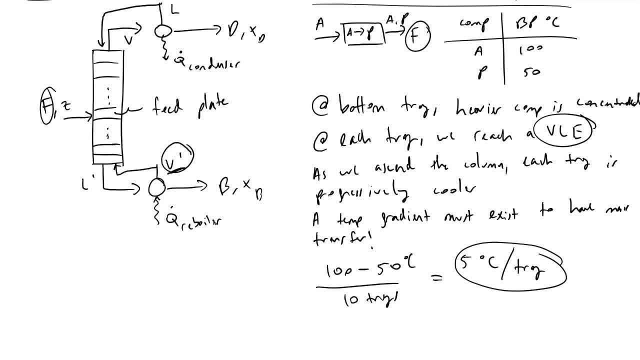 your lighter component, And this is V. So the vapor phase is concentrated in the lighter component, Which was our product P, And when we enter the condenser, as the name suggests, we're going to be extracting or removing heat from this stream, which is going to cause the incoming vapor to 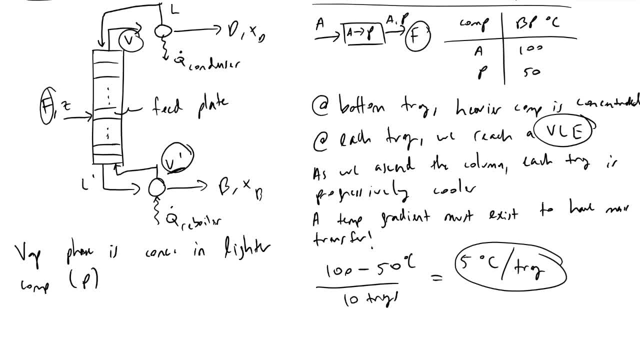 condense And we're going to get a liquid that will be rich in our product P, that we can sell to market because it's now purified And we can divert some of the liquid back down the tray or back down the column if we wanted to get better. 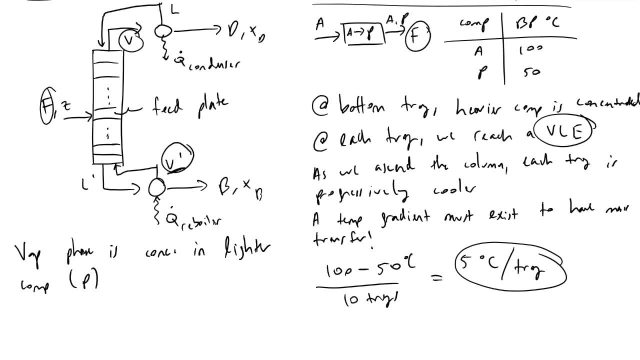 performance, And there are mathematical models that tell us what kind of ratio we want to have of sending that liquid back down the tray, And that is referred to as a reflux ratio. And so reflux ratio is one of the key parameters that chemical engineers adjust in practice. 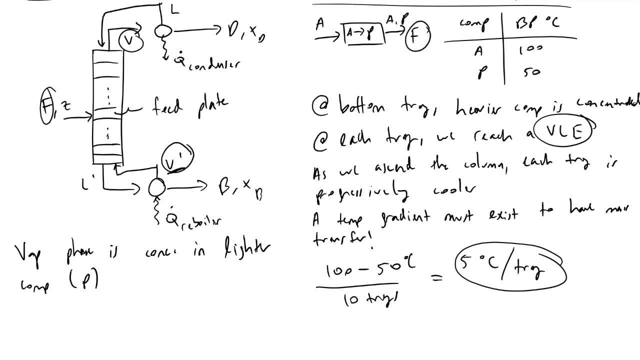 And I have other videos that discuss that, but this is an introduction, And so what we'll find is that the distillate has a mole ratio of the lighter component that is greater than the feed mole ratio, And so this is the take-home message of a distillation column. 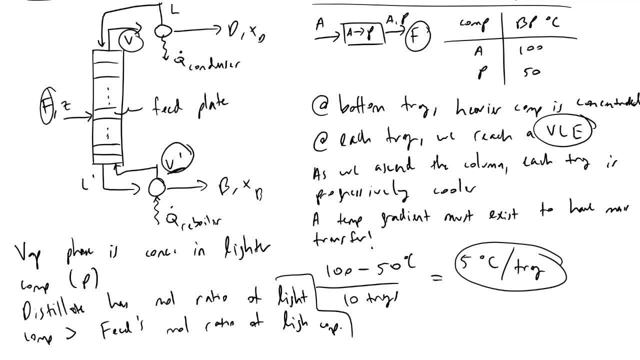 And we ended up with a distillate stream that has a product we can sell to market. And we also have this bottom stream here that we can send right back into our reactor to get better conversion of our reactants. And an important note: 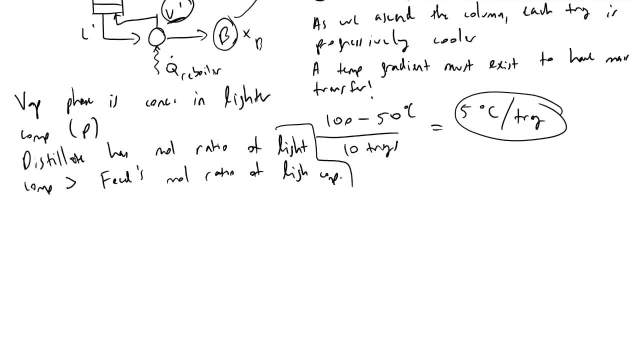 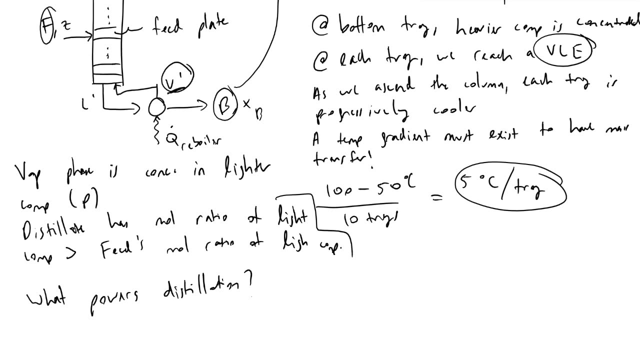 what we want to make here is what's powering distillation. In other words, if I wanted to double the amount of feed that I could send to my distillation column, if I wanted to make more product or purify more product, what parameter do I have to change? 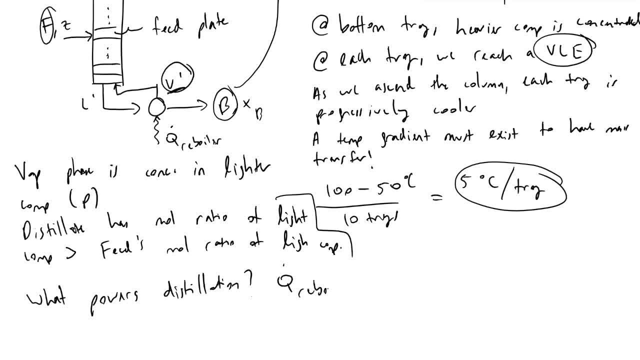 And the answer to that is Q- Reboiler. And so if we are doubling the mole flow rate that we're processing, we're going to need to double the amount of heat that we're supplying in our reboiler to vaporize. double the number of moles at our bottom plate. 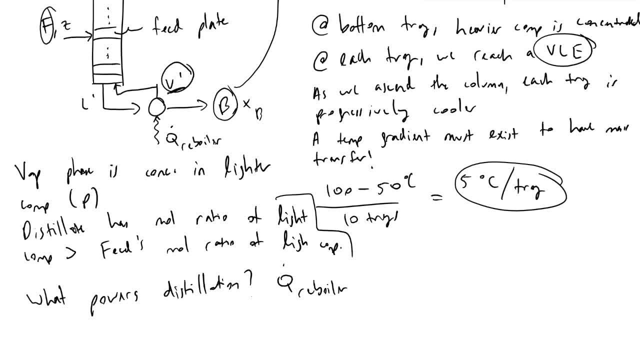 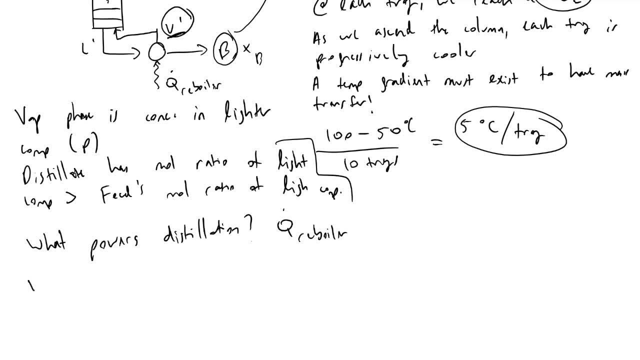 And this is how distillation works. And then a final note is, in terms of sizing, What should your distillate flow? What should the flow rate be, In other words, the letter D which denotes the mole flow of your distillate. 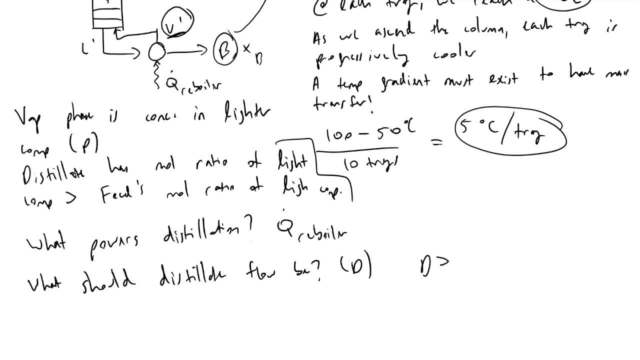 Well, we want to make sure that D is at least as big as the flow rate of our more volatile component in our feed stream. In other words, if we say, well, this is the total ratio, this is the energy, this is the demand, this is the demand, this is the flow. we're going to have to reduce it a little bit. So that's what we want to make sure we're doing. And if you're a separate company- let's say that you're out of rate- you're going to have to set up a medium of flow rate. In other words, if we have a gas feed that is already full, we're going to have to make sure that our distillate flow is going to be small. 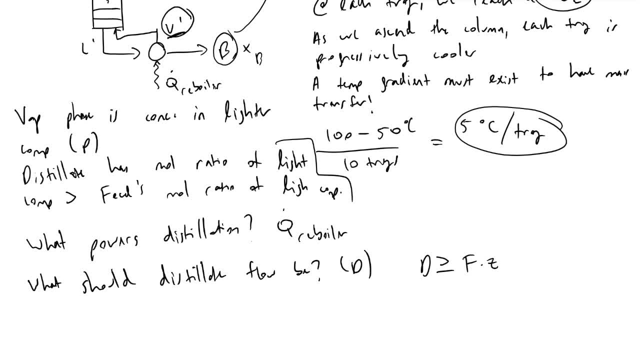 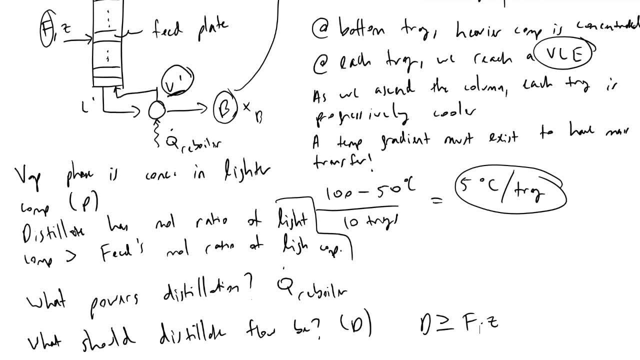 Let's say we have a single ratio of heat. if we had 50 moles of our product, which is a light component, entering our distillation column, we want to make sure that our distillate is at least as big or has at least as big of a molar. 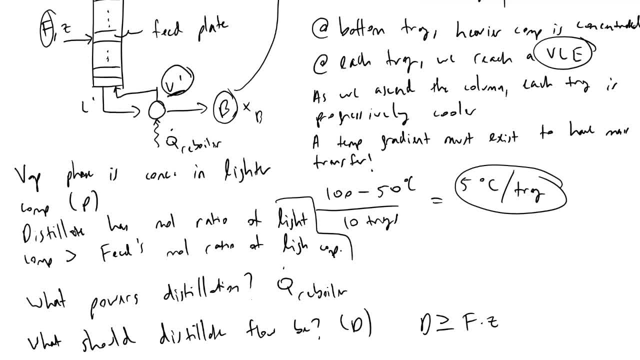 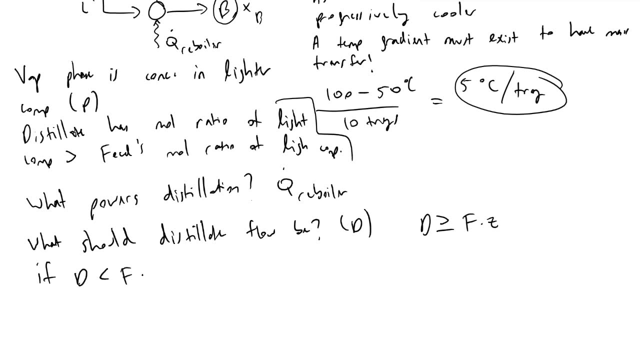 flow rate as our light component p. and the reasoning behind this should be intuitive, because if our distillate is less than the mole flow rate of your lighter component, so f is the total mole flow and z is the composition we get, accumulation of your product, which is the light component. 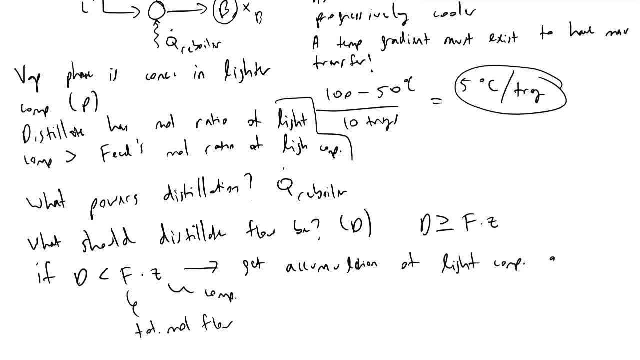 we want to remove the light component and lose the light component unnecessarily in the bottom stream. so you're sending your product back into your reactor and you're going to be getting a worse conversion because you're ruining the equilibrium condition inside a reactor. so it's a very tight looping process. so again, it's really hard to do without a drill.